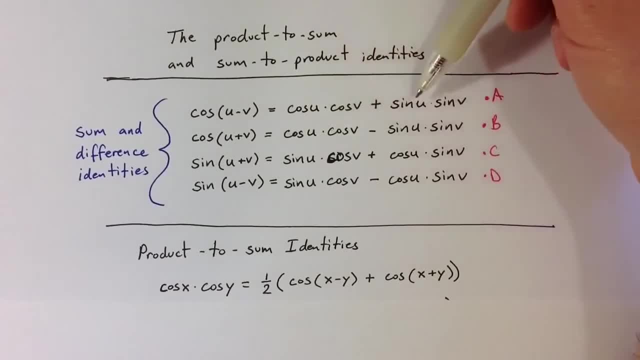 the sum. identity for cosine. The other term is sine of u, sine of v and minus, sine of u, times, sine of v, And so if we add those together, if I add identity A and identity B, the second term, the sine term, cancels out. 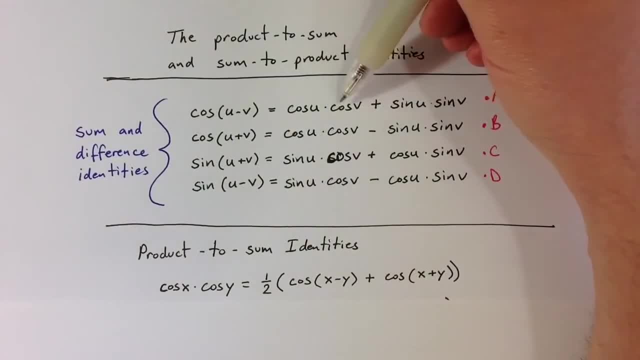 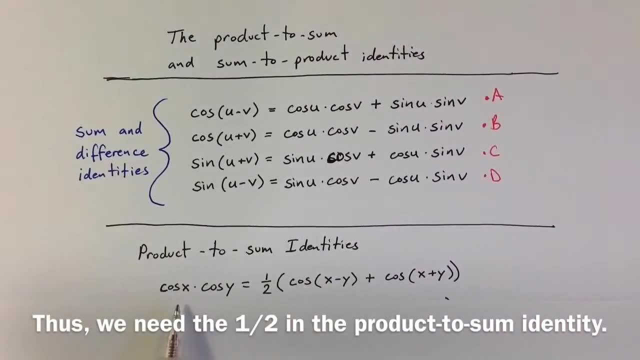 and we're left simply with cosine of u times cosine of v, but when we add those together we get two of them, And so changing the variables a little bit, but still it represents the same thing. variables are just placeholders, changing the u to an x and the v to a y. 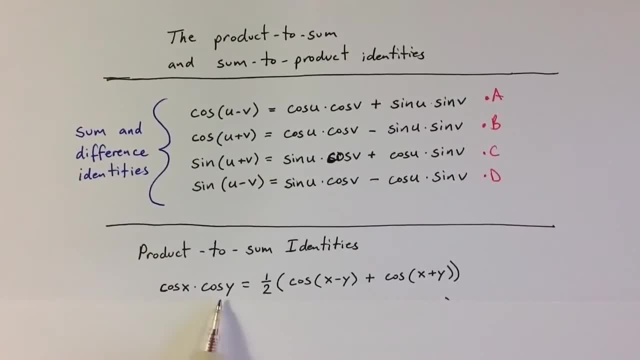 I get an identity that says: cosine of x times cosine of y is one-half the sum of cosine of bu minus v. so this is like the identity a up above. and cosine of x plus y- sorry, cosine of x minus y and cosine of x plus y. so this is like the identity b. 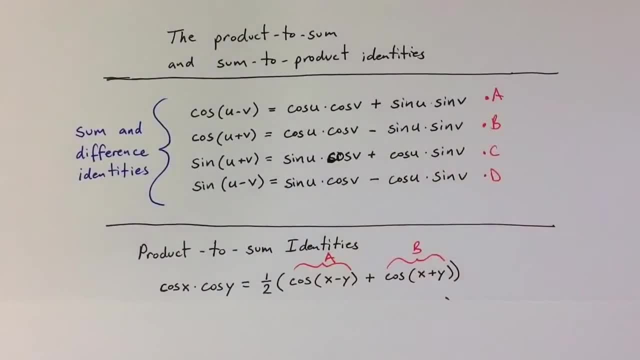 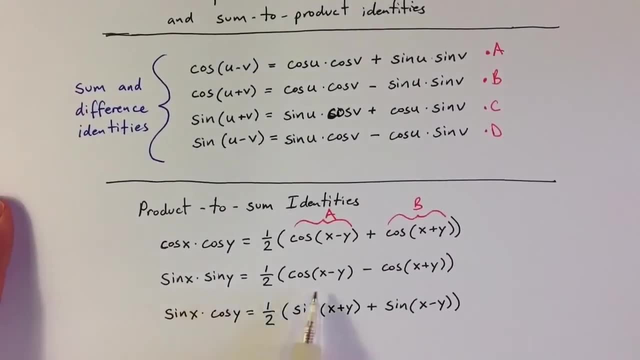 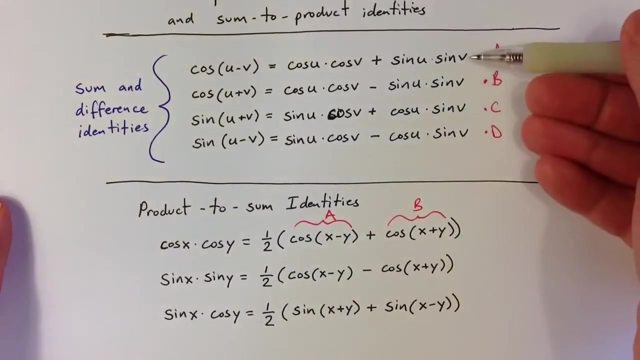 from above. in a similar way i can create a product to some identity for sine of x and sine of y by taking the identity a from up above and subtracting the identity b, because then the sine terms remain, but the cosine terms disappear, and so the product of sine of x and sine of y is one half. 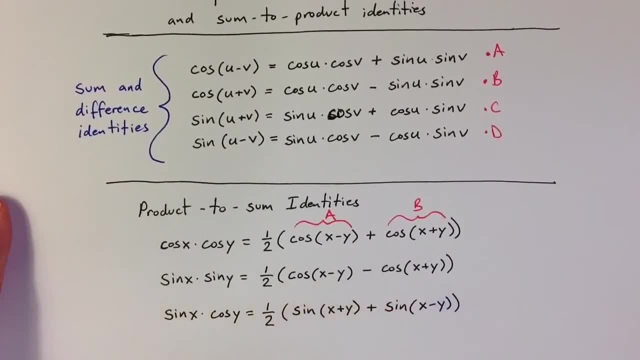 cosine of x minus y minus, cosine of x plus y. to get a mixed product with sine and cosine, we can simply add the second, uh sorry, the third and fourth identities c and d, because then this, the second term, will cancel here. cosine of u times sine of v, cosine of u. 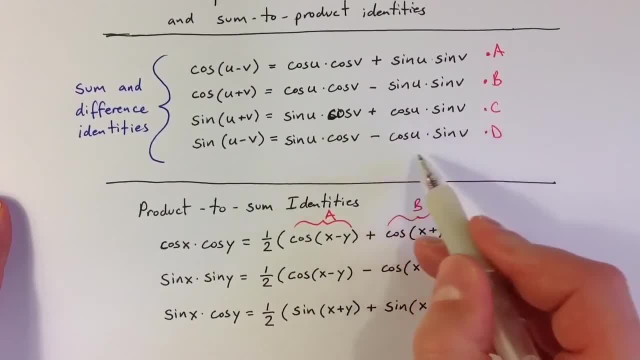 uh times, sine of v, one is positive, one's negative, so those disappear and we're left with sine of u cosine of v, sine of u cosine of v, and changing again, changing the u to x and the cosine or the v to y, we get the product identity for sine and cosine. 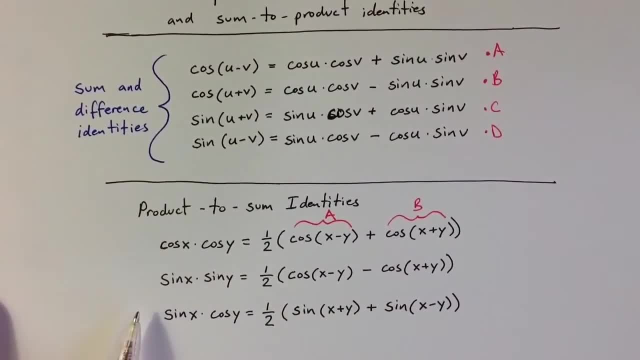 so these product to some identities are really useful in mathematics. changing a product into a product is really useful in mathematics. changing a product into a sum can be very helpful because in certain calculations, especially when you get into calculus, there are some things that we can't really do with a product. 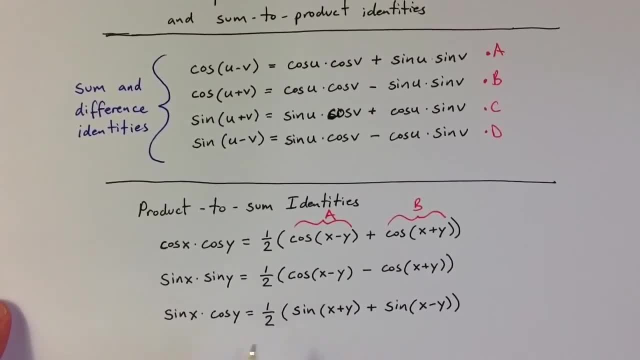 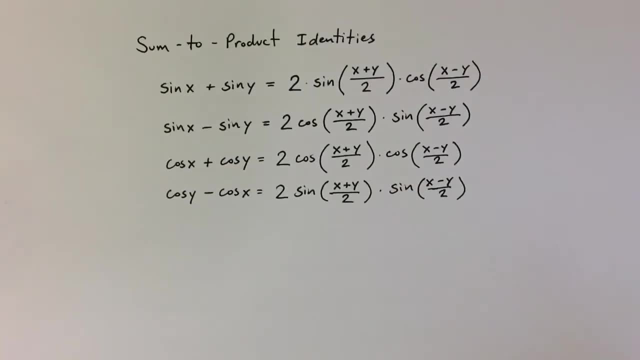 as easily as we can do with a sum and so changing a product into a sum uh can have some real advantages in calculation. also, from the sum and difference identities we can develop sum to product identities. to do this it's a little bit trickier, but let me explain at least the setup of our first identity. 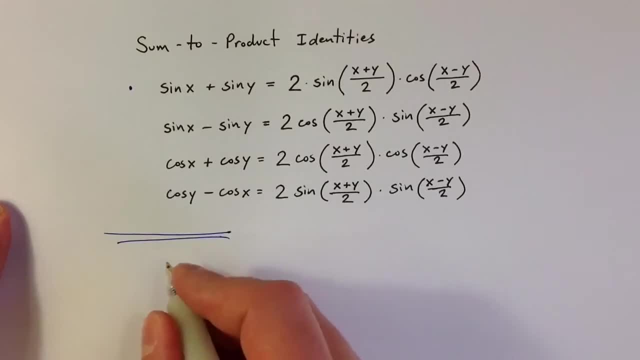 uh, sine of x plus sine of y. so what i want to do is think of sine of x plus sine of y in a kind of interesting way. uh, i mentioned in an earlier video that sometimes adding a form of zero can help us make progress in an identity, and that's the case here. 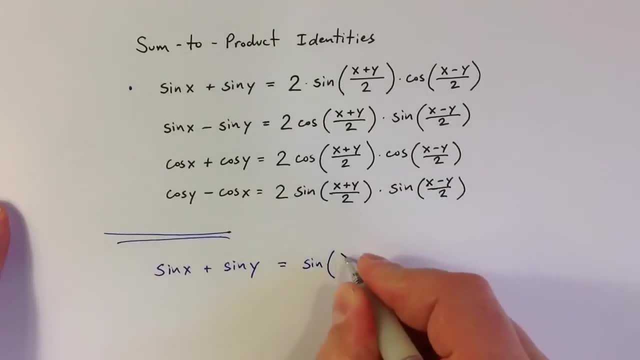 so what i'm going to use, since i never x into side of x over to plus y over two, plus xover two, minus way over two, until i added why over two? and took away y over two and i split the acts into uh, two parts as well, experts over to win y over two. 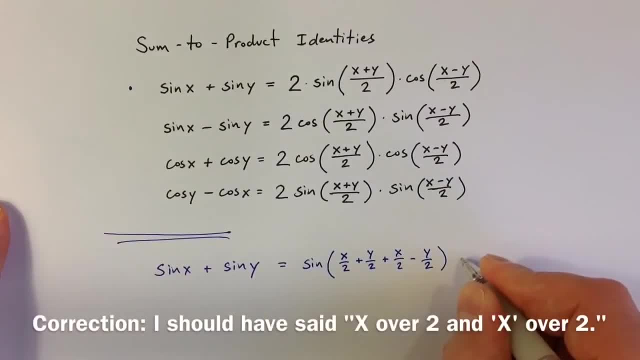 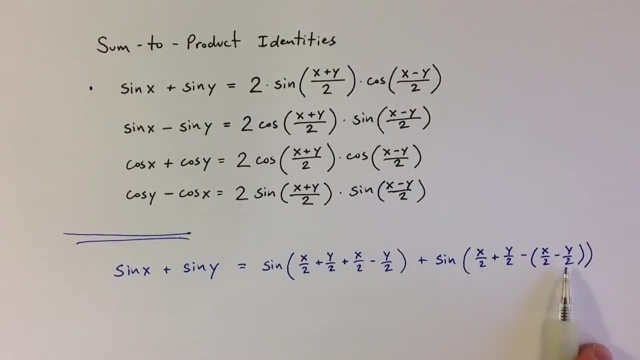 and i want a rewrite why- as sign of x over two- und Ask Williams earthquake- over 2 plus y over 2, minus x over 2 minus y over 2. so here the negative sign cancels the, the y over 2 and it makes it a positive. 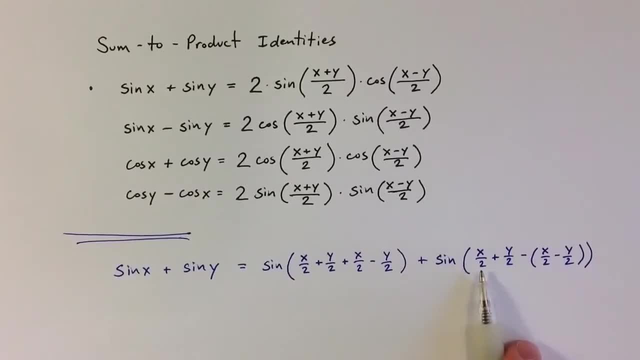 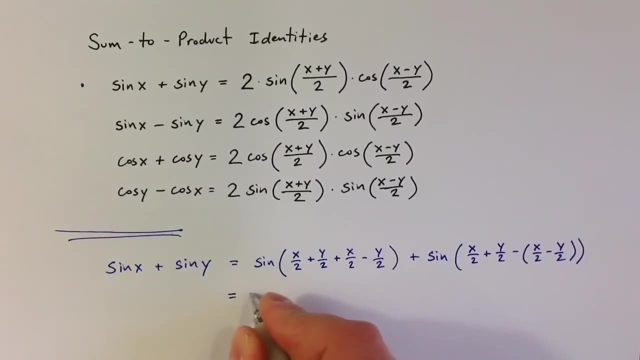 y over 2 in the end, but we get a negative x over 2 and a positive x over 2 that cancel out. the reason for doing that is that now I can group those so that I have sine of x plus y over 2, plus x minus y over 2. 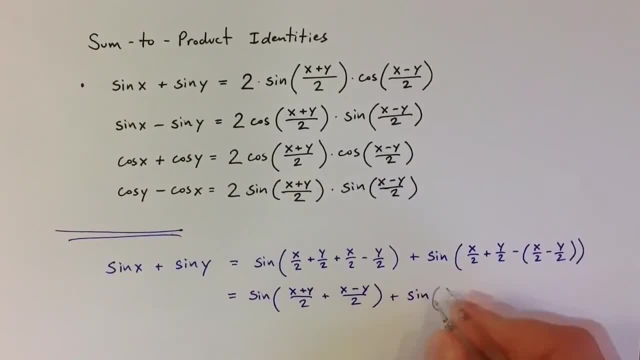 plus sine of x plus y over 2, minus x minus y over 2, and then I can think of the sum and difference identities for sine. if I think of this as u plus v, my first expression, I can rewrite further using sine of u plus v.